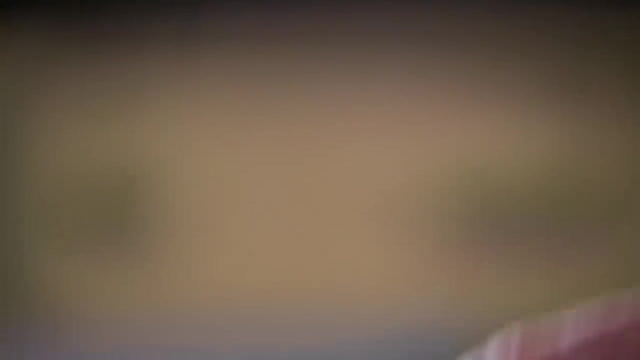 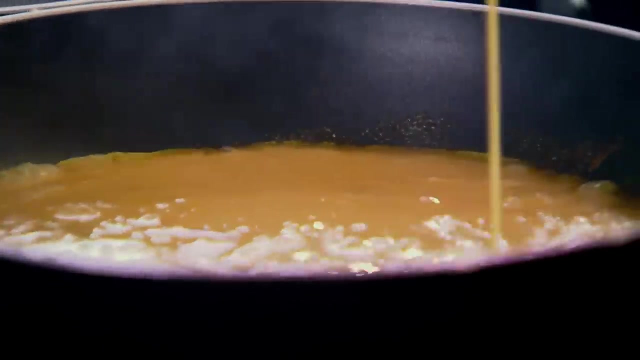 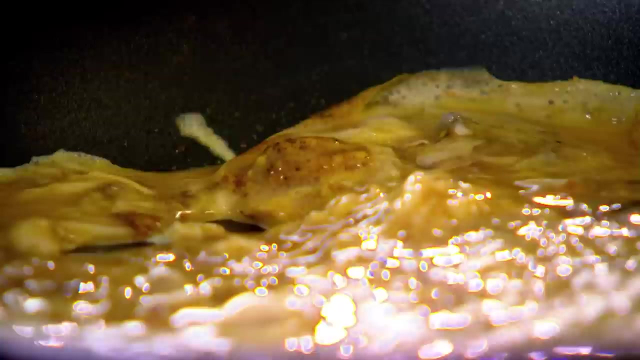 add a teaspoon of garam masala and turmeric. Cook that out Now take your eggs into the pan- Almost going to make like a really nice spicy scrambled egg. Turn the gas down Now as the scrambled egg comes together. just finish that with a little bit of butter. 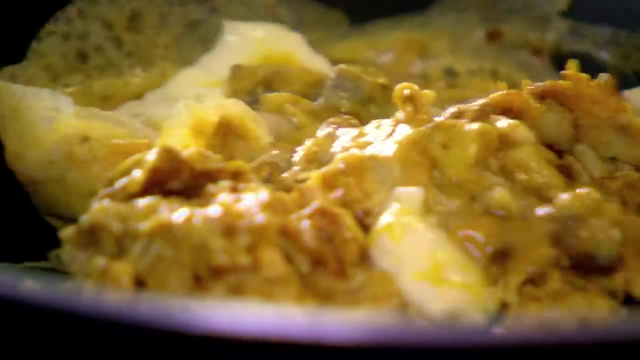 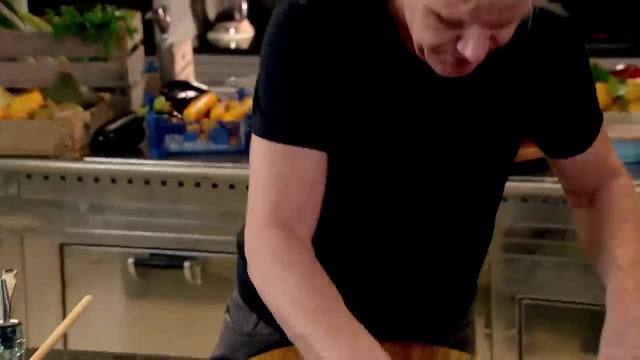 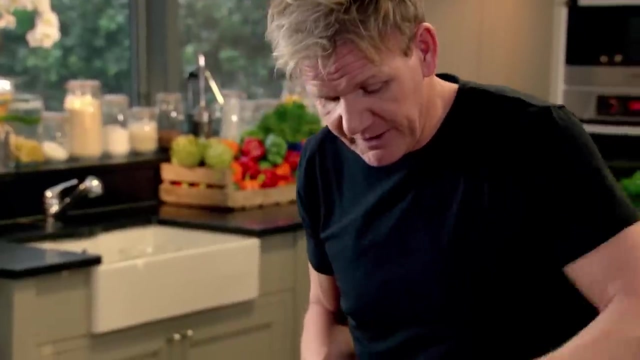 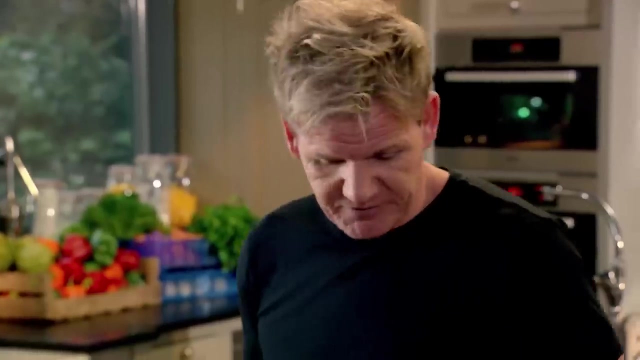 I quite like. the sort of creaminess Makes it so much more delicious. And then from there I'm going to get my spinach Chop up and then fold in The spinach to your scrambled egg- Something quite exciting about eating spice for breakfast. but it's served in these wonderful 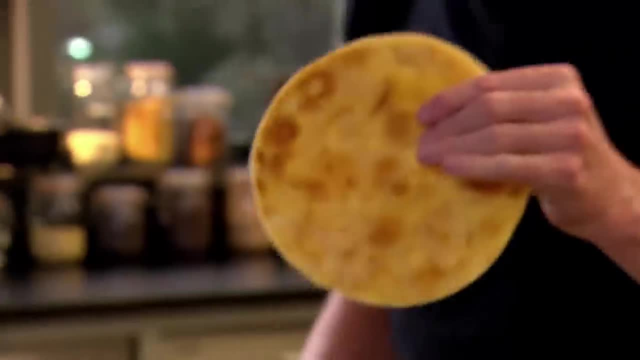 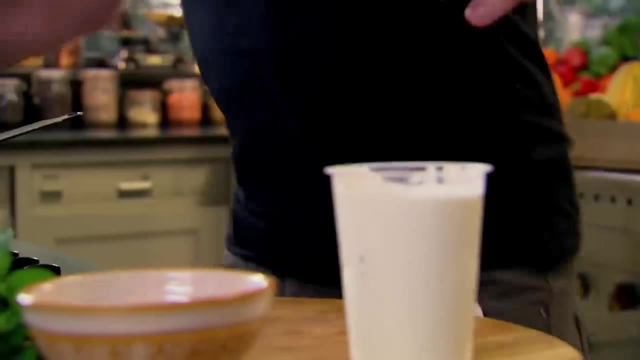 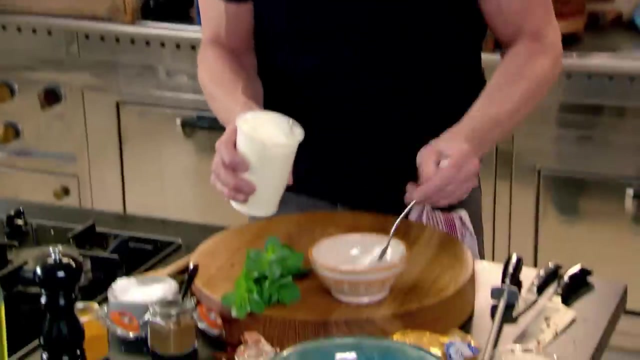 little thin naan breads. This will work with any flatbread or wrap you fancy And then lightly toast your naan. Take the eggs off the heat whilst you get on with the last job at quick mint and spice yoghurt dressing. Couple of tablespoons of fresh yoghurt in There's always something. 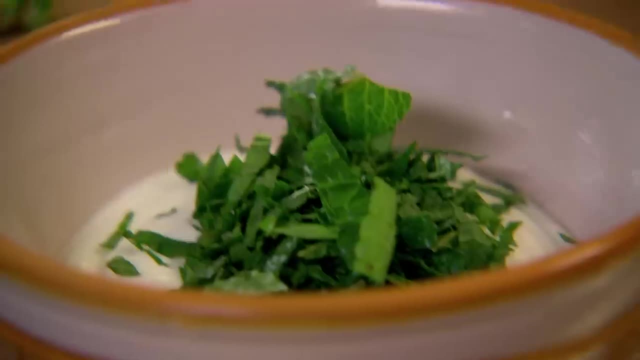 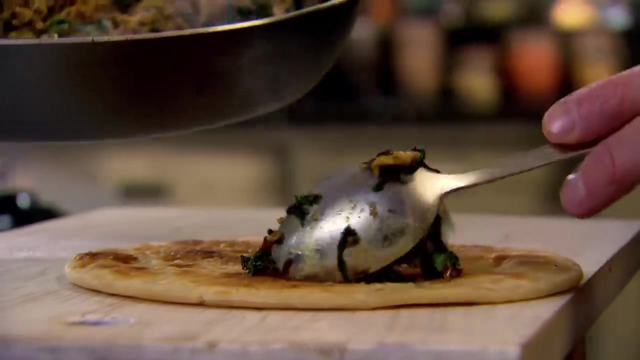 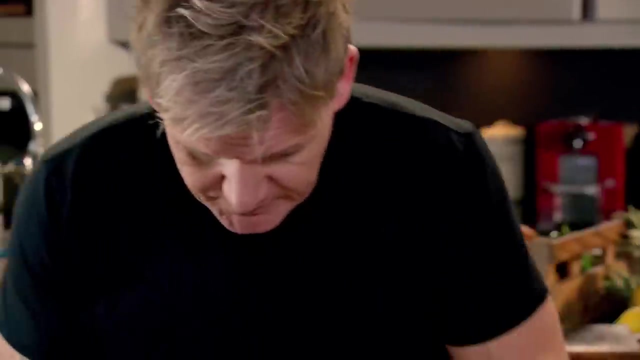 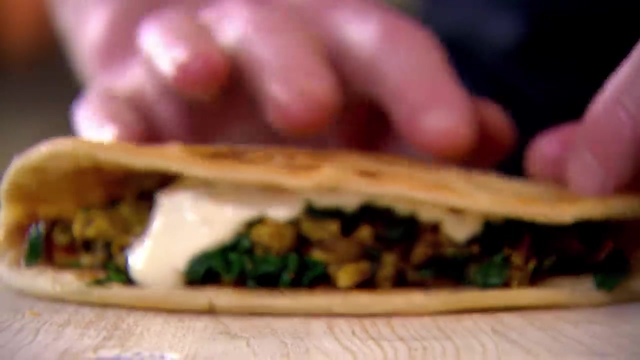 to take out the heat. Then add chopped mint, salt and turmeric Mix. that in. Now take scrambled egg and half fill of naan. It smells incredible. Get your yoghurt, Come that down on top and lift that over, And for me that's what really stands out with street food in India. 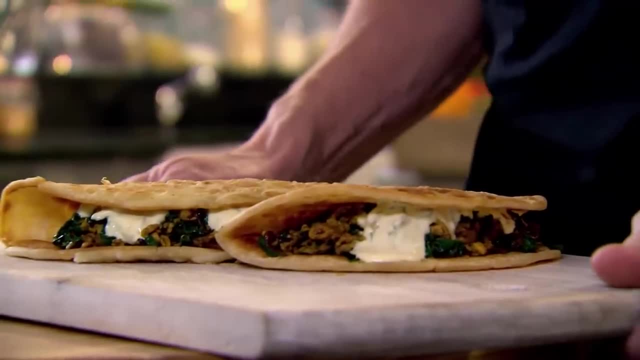 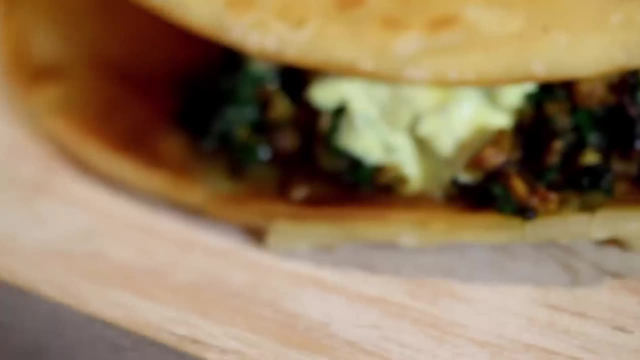 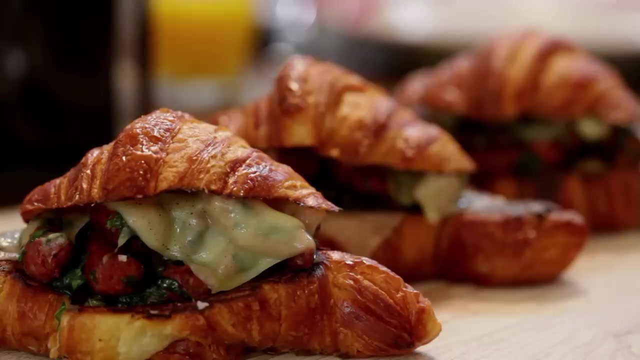 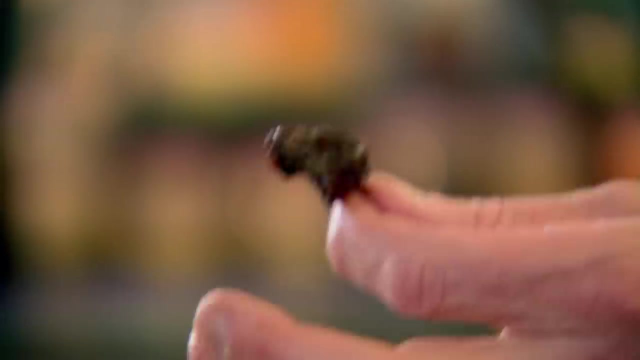 How delicious they can make street food with a little bit of spice. amazing. Once you try this spicy wrap, I promise you scrambled eggs will never taste the same. a Punchy breakfast of merguez and fontina stuffed croissants- Flavor there is incredible. for lunch, a spicy Mexican soup. be adventurous but beware. 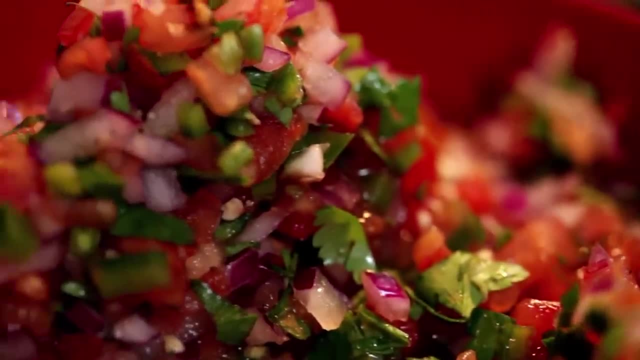 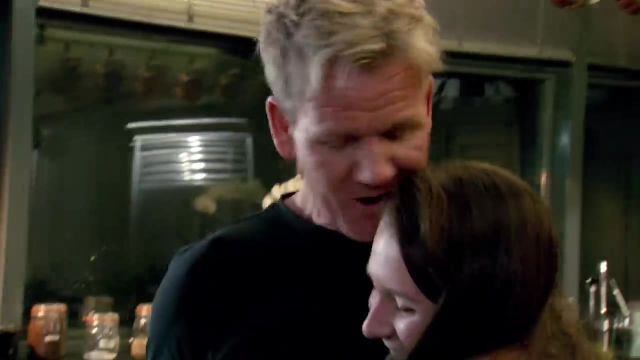 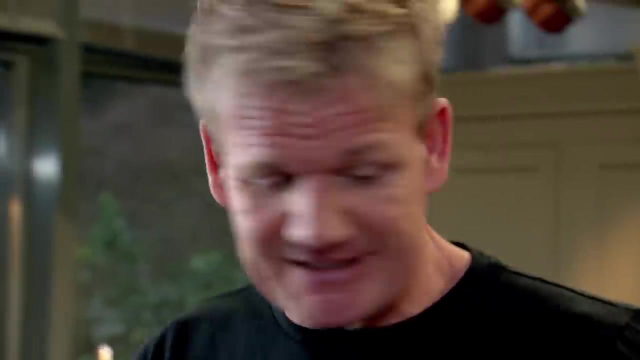 Serve with quick tortilla chips and a pico de gallo dip. May be for dinner. I'll be setting the world to rights with my eldest Megan When we make one of her favorite dishes: crispy roast duck with pancakes and black bean dipping sauce. Seen as is your favorite. now you can make it, followed by a spiced banana tart to tan- Wow. 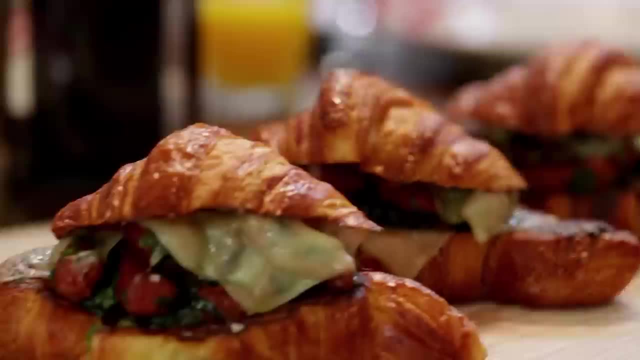 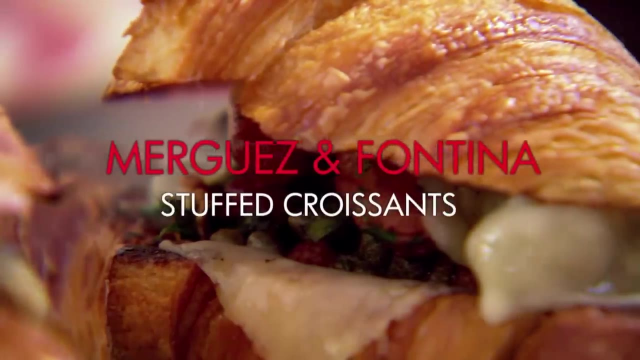 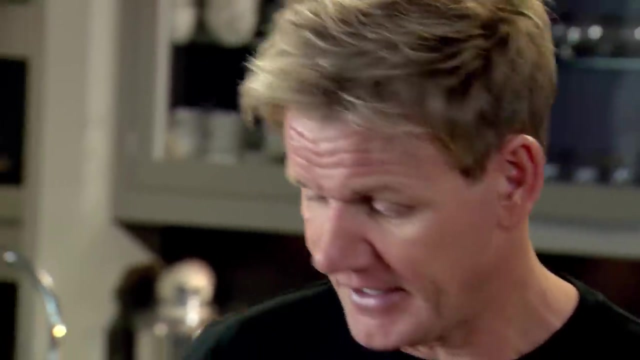 These are my ultimate recipes for a day bursting with a big and bold breakfast, lunch and dinner, starting with a breakfast That can't fail to wake you up: merguez and fontina stuffed croissants. Okay, big and bold. I was living in France. I stayed there for three years, once, twice a week. 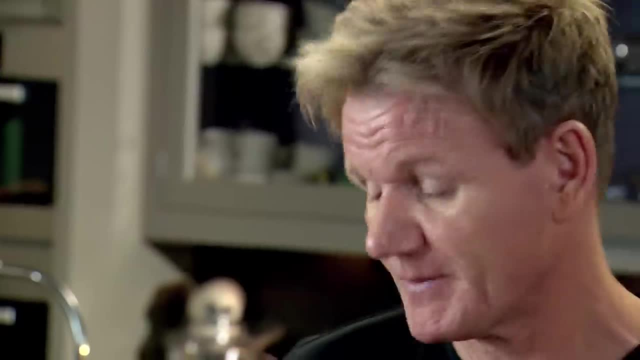 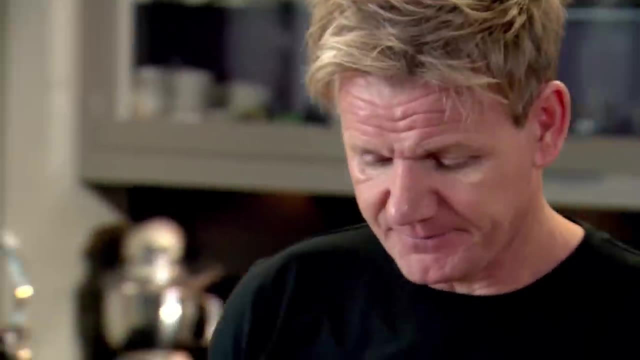 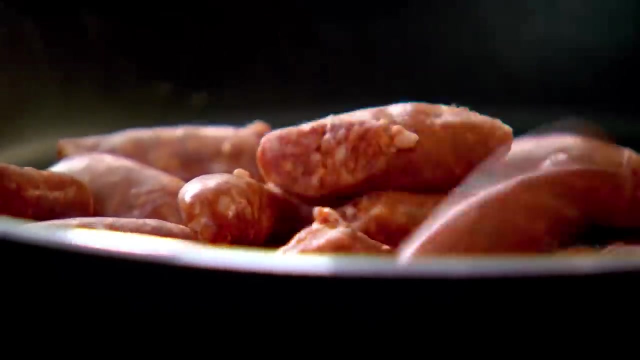 I treated myself to the most amazing Bold breakfast and it started off with these beauties here: merguez- cheap but incredibly tasty. Start off with a nice hot pan. merguez in. It's a very spicy sausage. doesn't need any help to be the chili, just a touch. 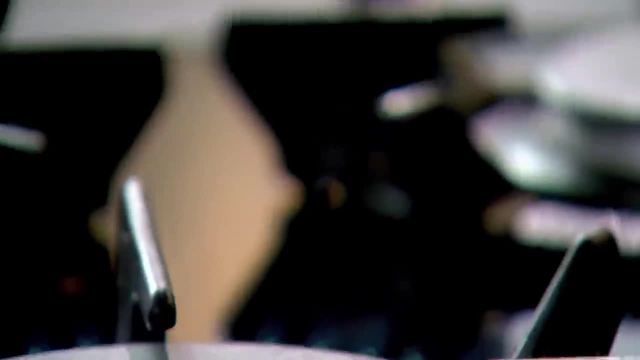 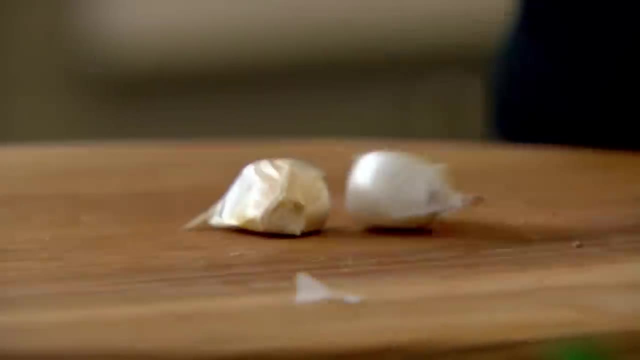 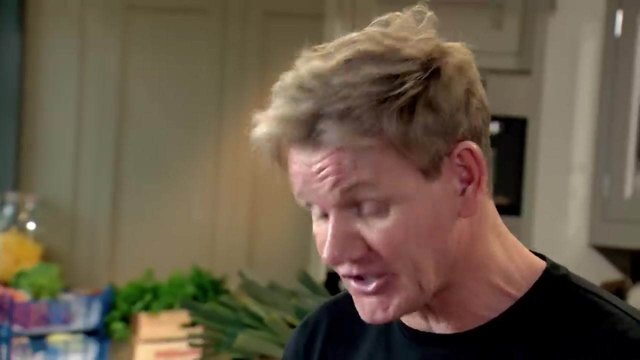 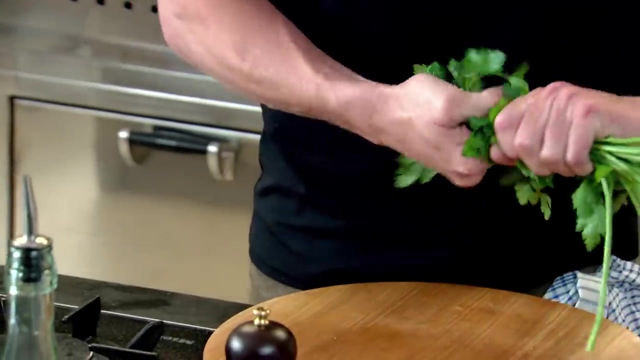 of salt and pepper. You can smell the spice. they're starting to release all that wonderful oil, that flavor, in there. Add a couple of cloves or finely sliced garlic. Spread the garlic across the pan. it instantly changes color, takes on this nice, dark, rich golden color. Now take a look with the heat out for the parsley. 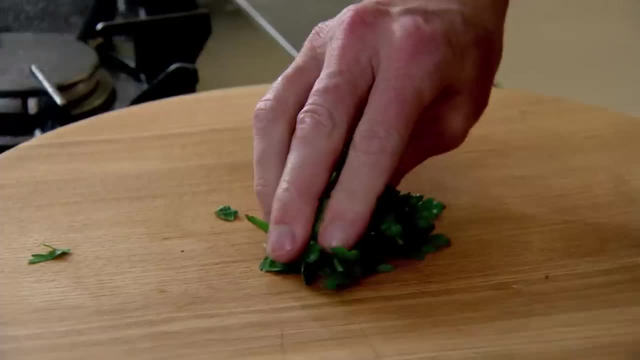 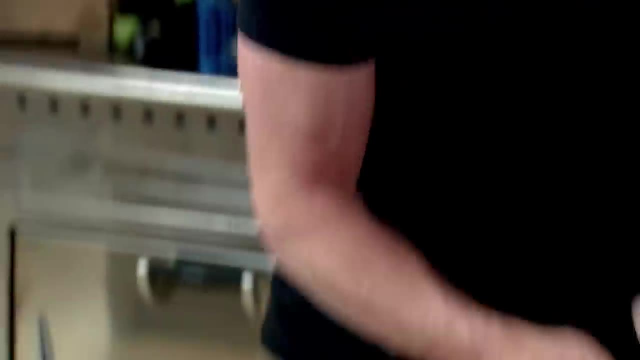 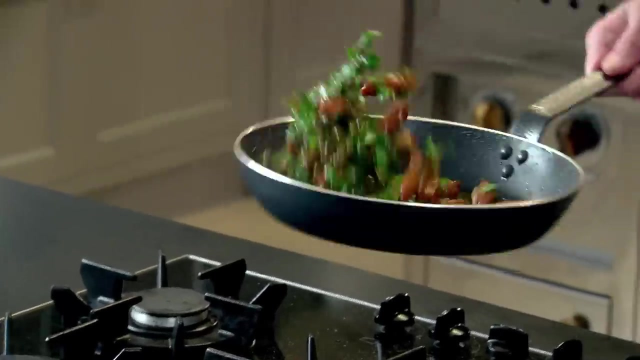 the stalks of soft herbs like parsley and coriander can be used to impart Flavor during cooking, but the leaf should always be added just before serving to give maximum color and fragrance. And then finish that off with my capers. Now take your croissant. 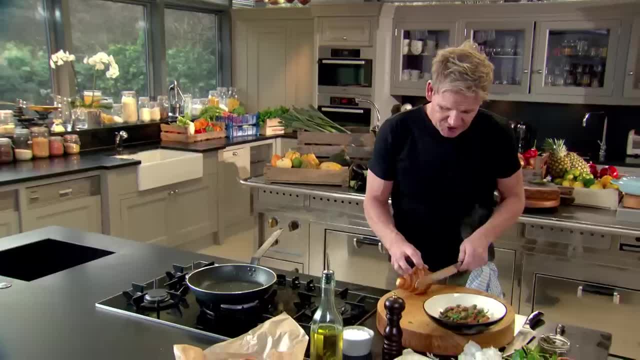 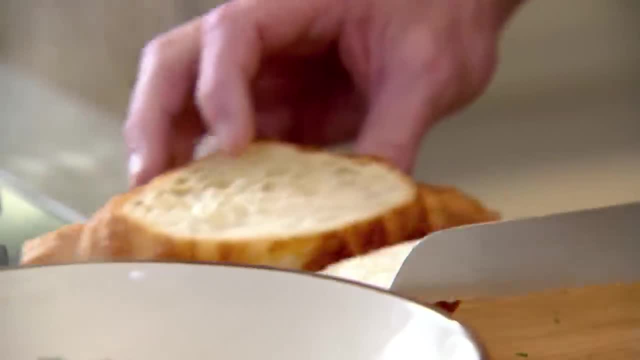 They're literally 24 hours old, so they're crispy on the outside and just slice off the lid. This recipe is a great way to use up any leftover croissant from the day before. I Used to cringe when I saw the French cooks throw away croissants. I used to cry thinking, oh my god. 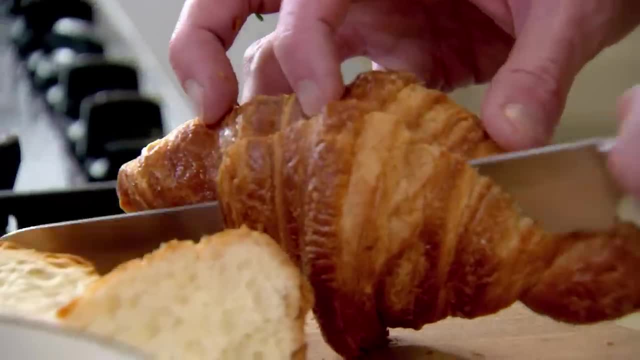 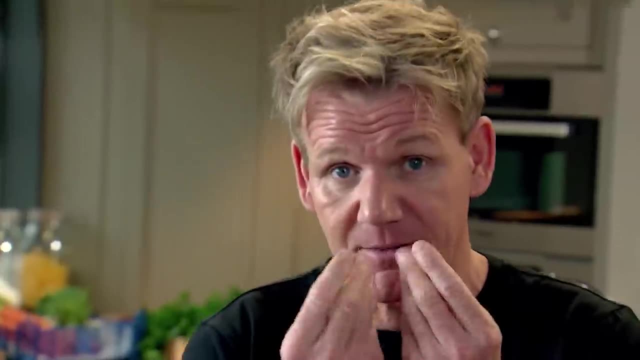 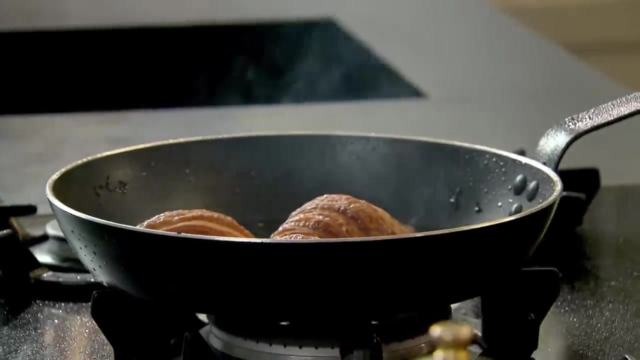 Any idea what you're throwing away in terms of flavor. Whatever you do, do not wipe out that pan. dunk your croissants, mopping up all that amazing flavor and caramelizing the inside for that beautiful, and don't forget the lids. And then get your thumbs and go inside the croissant. 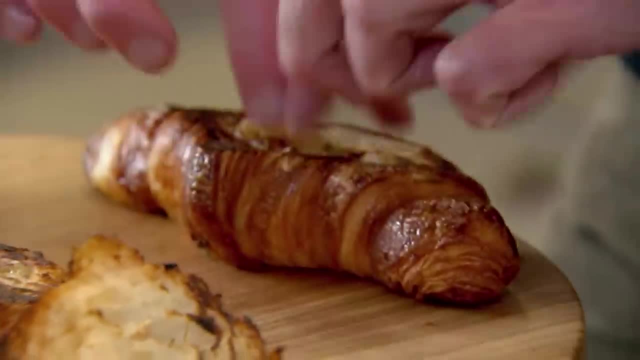 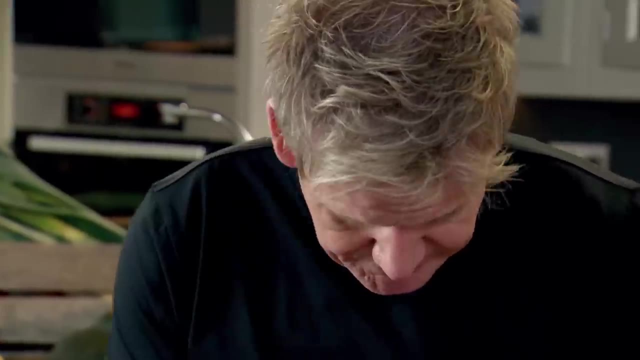 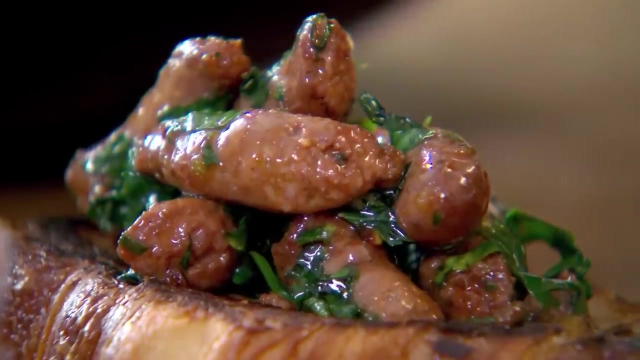 All I want to do now is just create a little pocket and just manipulate the croissant. now This is where it gets exciting. Mix up the capers, the garlic and sausages. Look at the color of that wonderful, Delicious flavored oil. now some cheese, but not just any cheese. 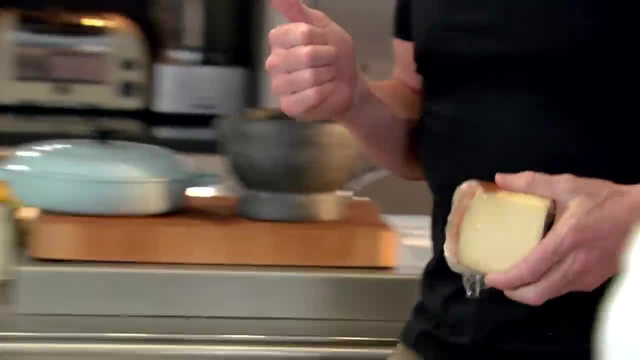 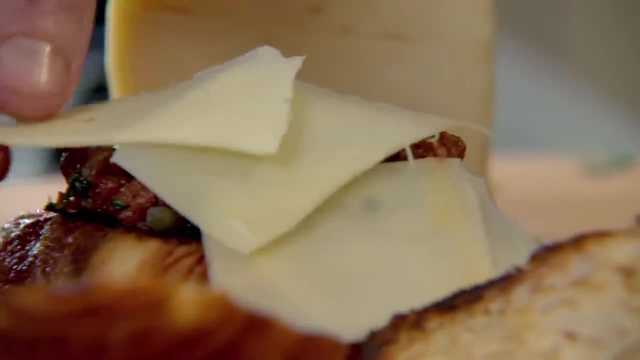 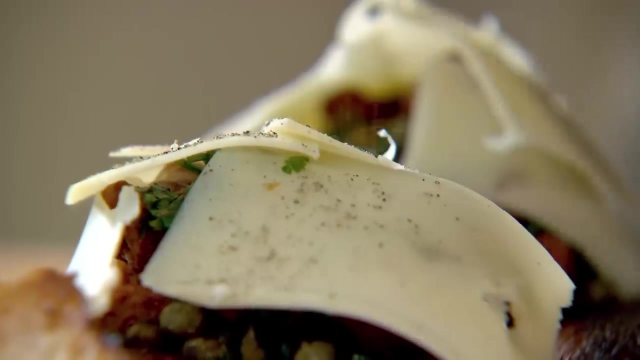 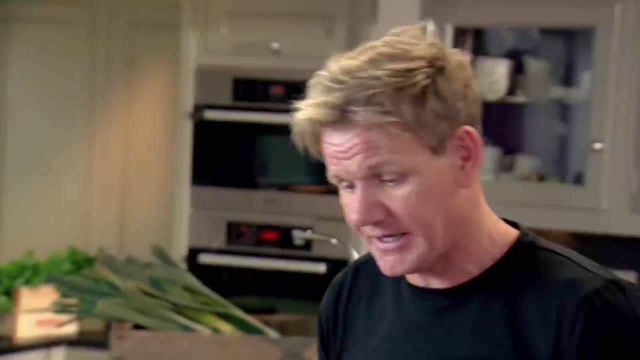 Fontina cheese is like the number one cheese for grilling and because it's a very rich cheese you shave it thinner And you would a white truffle, but it gives a really nice saltiness and a light smoky flavor. Touch of pepper Salt. place these big boys on the tray, literally 30 seconds on the grill. 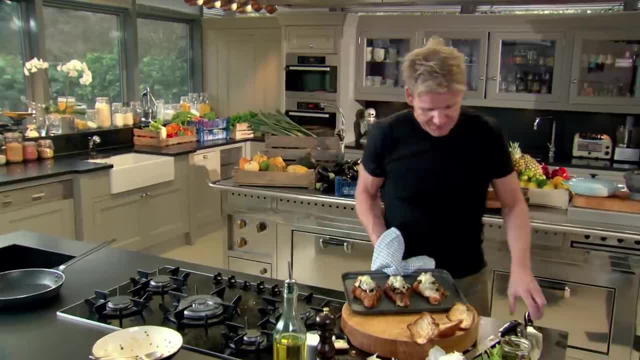 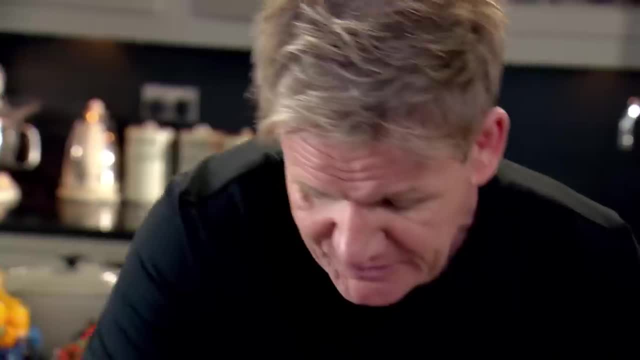 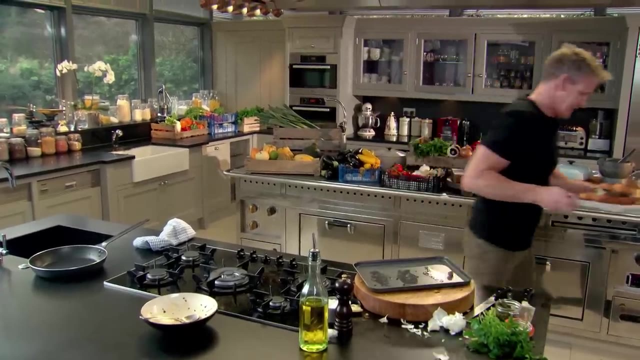 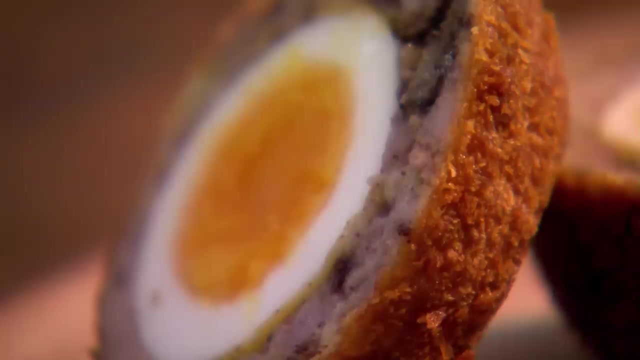 Here we go. nice crisp packs full of flavor. now Top them, and that for me It's almost like being back in Paris, Except this time I don't have to share them with the French. My ultimate big and bold breakfast: merguez and fontina stuffed croissants, the perfect picnic breakfast. my ultimate scotch eggs with a twist. I. 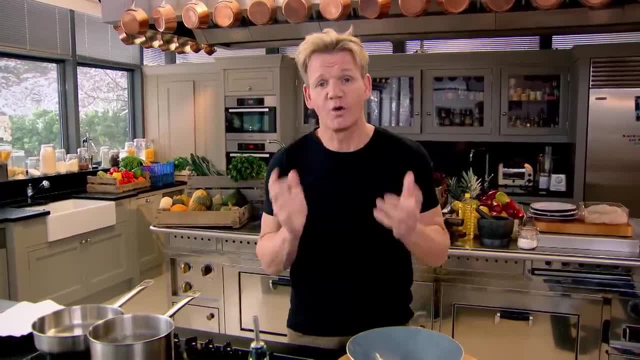 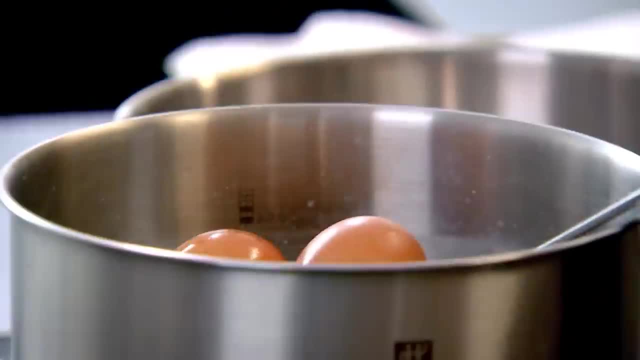 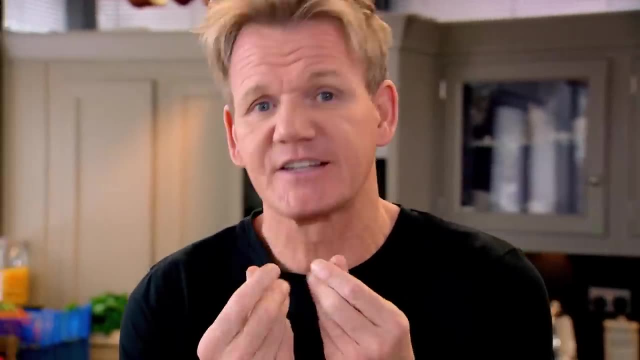 Go fishing a lot and scotch eggs are the perfect all-in-one mini picnic breakfast. first thing, get your eggs cooked, Bring the water up the ball onto the spoon and lower them into the water. that way they don't hit the water and crack. Four and a half minutes that will keep the center nice. 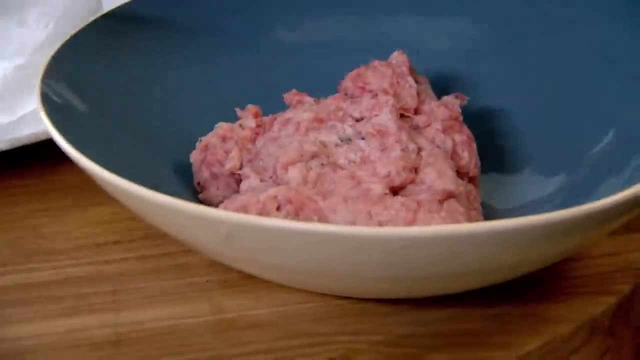 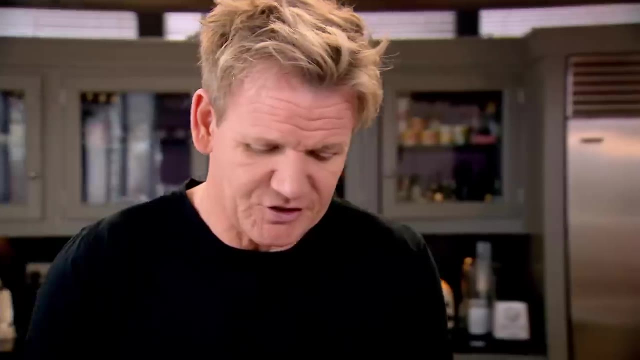 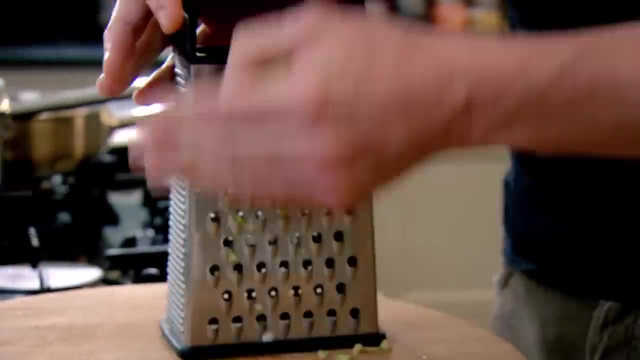 Slightly running now ground sausage meat. I'm gonna make mine a little bit spicier. I'm gonna crumble in black pudding that helps to season scotch eggs inside a little touch of salt and pepper And then just to make it a little bit sweeter and a lot easier for the kids to eat, some grated apples. 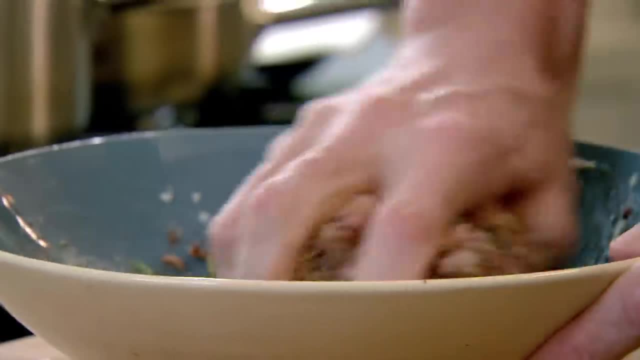 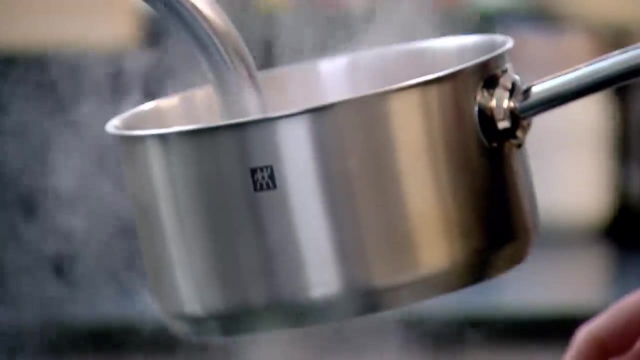 And then just to make it a little bit sweeter and a lot easier for the kids to eat, some grated apples. Combine that blend in the apple and the black pudding eggs. once they're cooked, drain them and then run them under cold water. Cracking and cooling the eggs quickly will prevent the yolks turning gray. 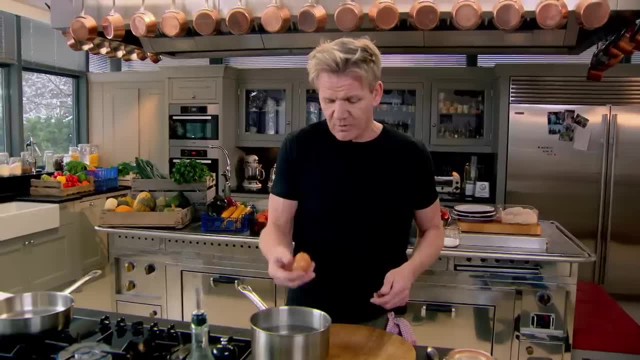 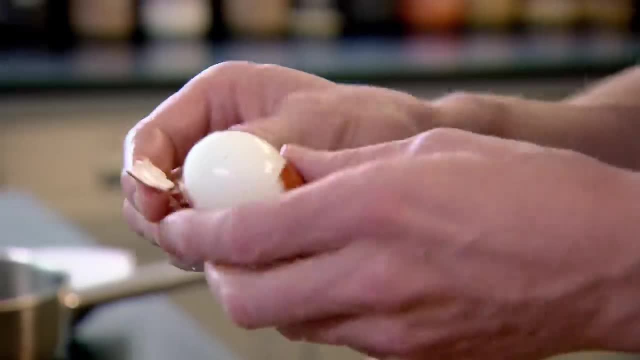 Tap them on the side of the pan, put them back into the water and what happens? the water seeps underneath the shell. See the shelf come off. so much easier. eggs still slightly softened: Center on that little bit of richness with the yolk. Next you need to get yourself organized. 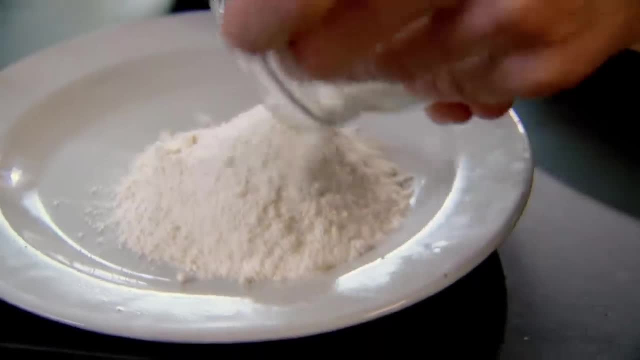 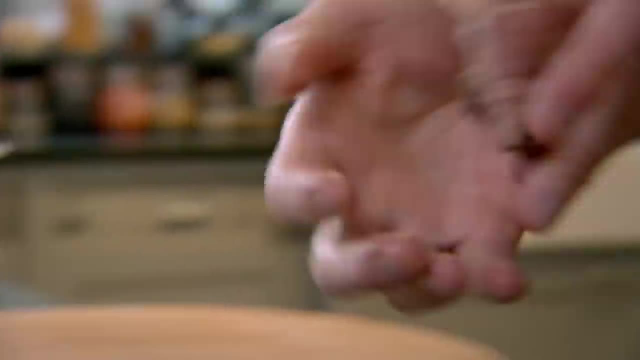 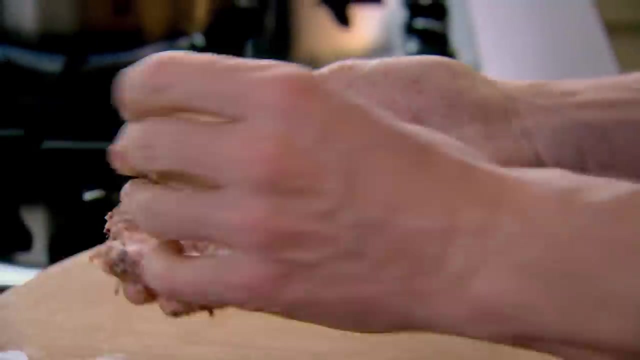 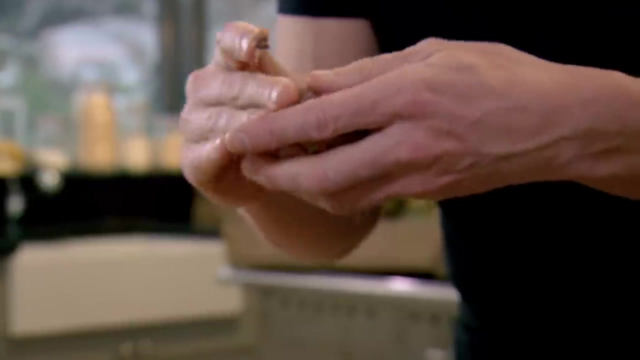 with a mini assembly line: seasoned flour, a Little egg wash And breadcrumbs. take your mince golf ball size, Spread the pate, manipulate with your thumb and then sit your egg in there and spread the sausage over the egg And you just seal that over. Really important to keep that nice. even coating of sausage meat around the egg. You don't want it too thick. 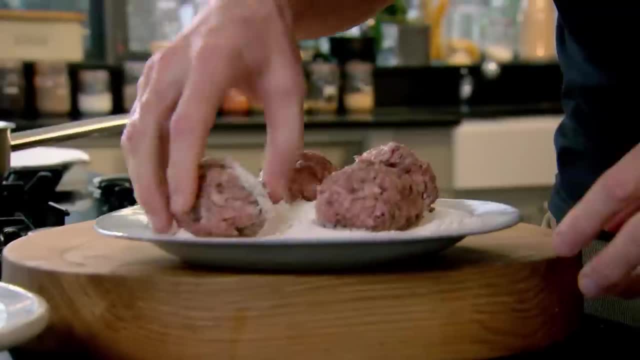 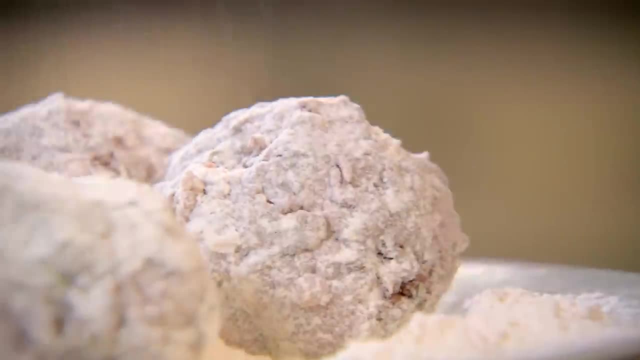 Otherwise it gets too dense And it's unappetizing. give them a light. dusting in the seasoned flour. If you don't put the flour on the egg wash won't stick. if you don't put the egg wash on the breadcrumbs won't stick. 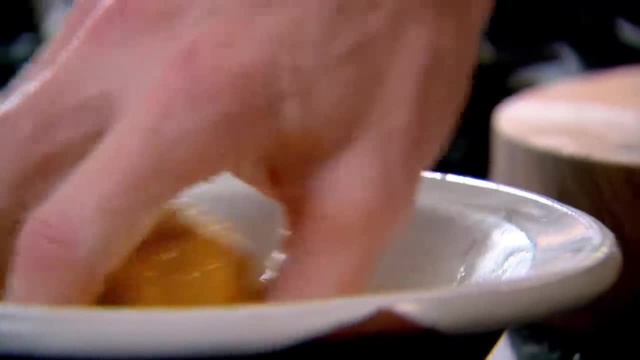 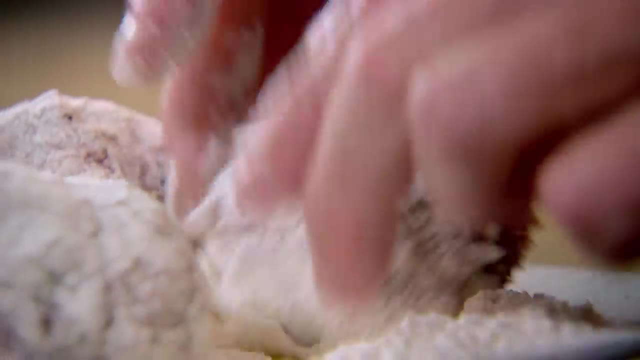 into the egg, Roll it round, Shake off any excess egg wash and roll it into your breadcrumbs. You can use this same three-stage method to breadcrumb anything you'd like, from chicken goujons and fish fillets to pina schnitzel. These are panko breadcrumbs, Japanese. 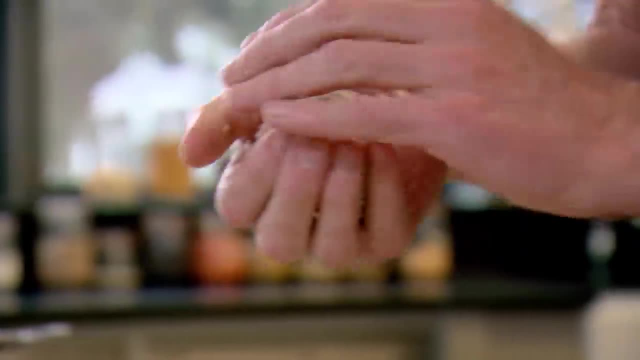 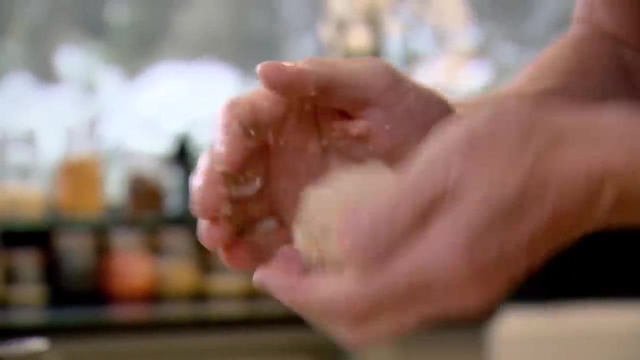 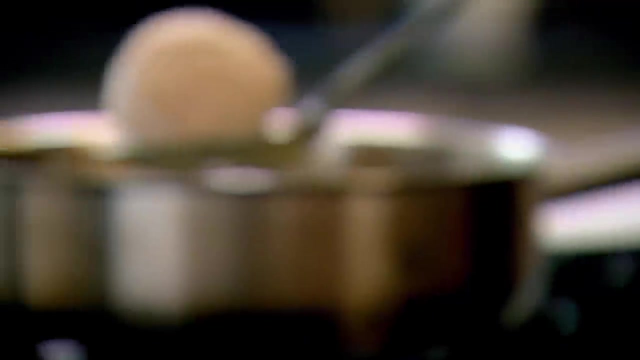 White breadcrumb, so no crust. You can experiment by adding flavors to your breadcrumbs, like parmesan herbs or citrus zest. I always like to push the actual breadcrumbs into the sausage meat so it gets that really nice golden brown and stops any the outside burning. Once breadcrumbs know the eggs carefully into a four centimeter deep bath of hot vegetable oil for 10 to 12 minutes. 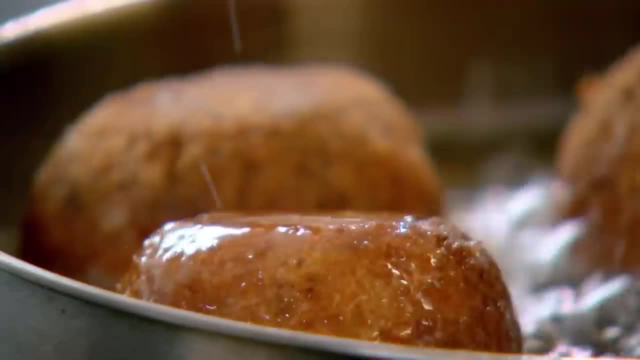 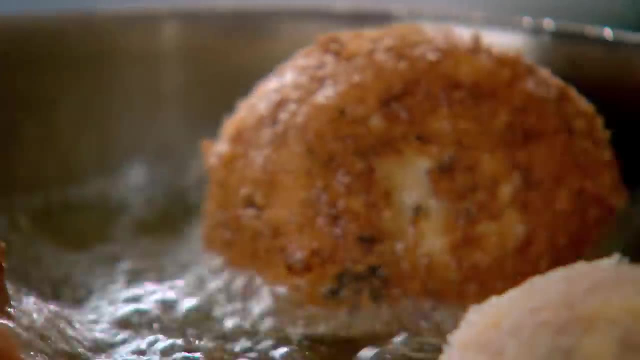 The eggs are actually cooked soft and running the center, So the objective is just to cook the sausage meat and the black pudding. Look great, don't they? Little egg grenades. There's something so magical about a scotch egg on a picnic because it's like this little mini breakfast. 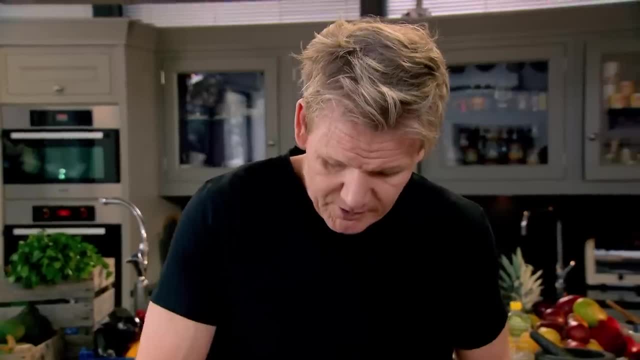 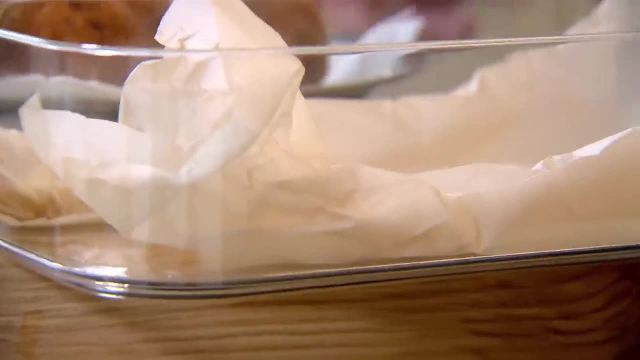 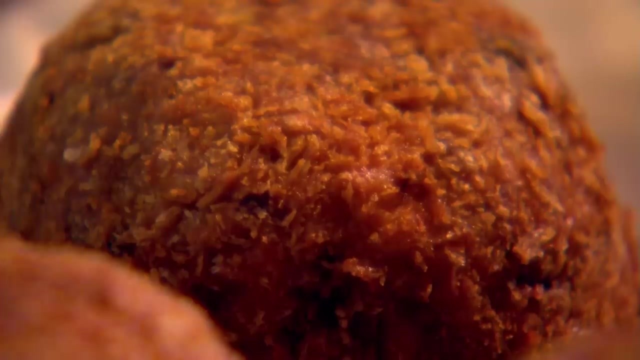 beautiful, Drain them onto the paper, roll them around Just to get off any excess oil and then to transport them. some greaseproof paper- That for me is the perfect start to the fishing trip. There's no wonder I never catch any fish, because I'm always too busy eating my scotch eggs. 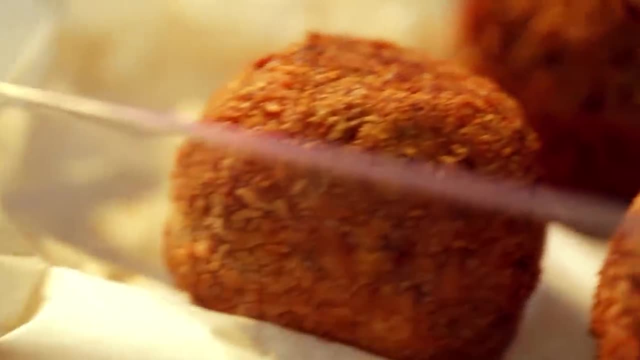 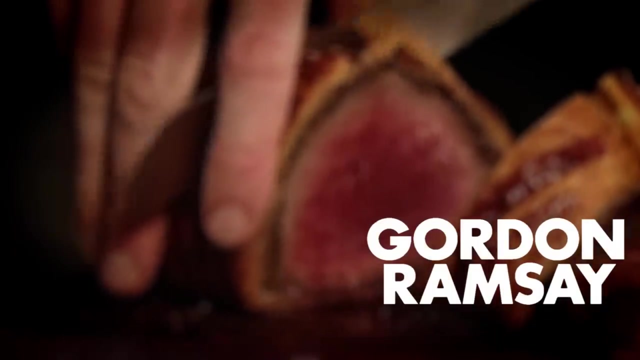 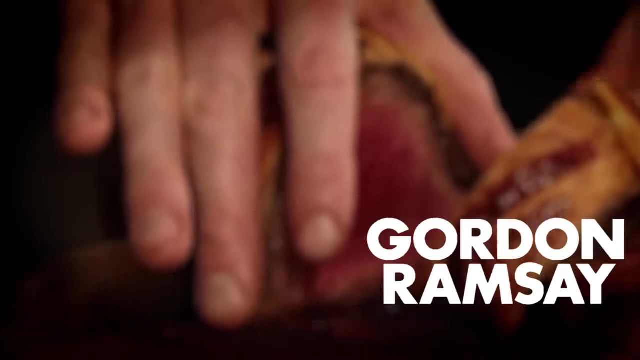 My ultimate black pudding lace scotch eggs, an irresistibly delicious picnic breakfast. You, You.